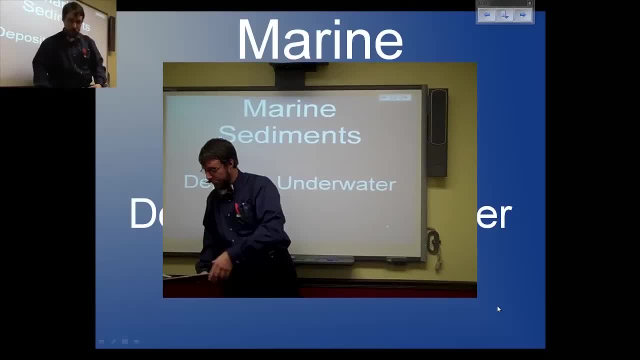 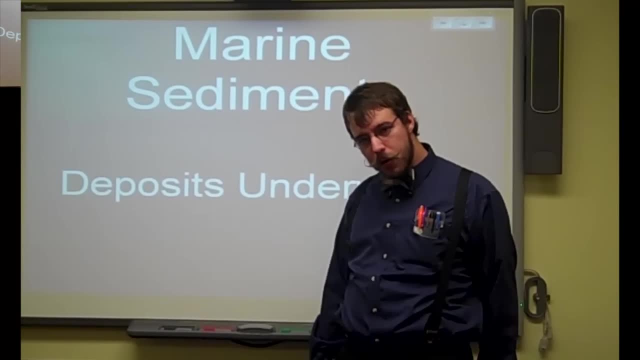 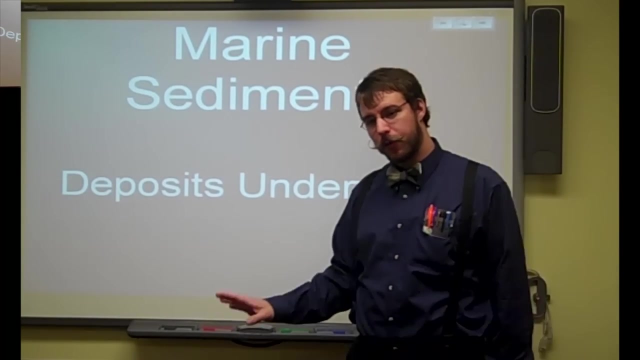 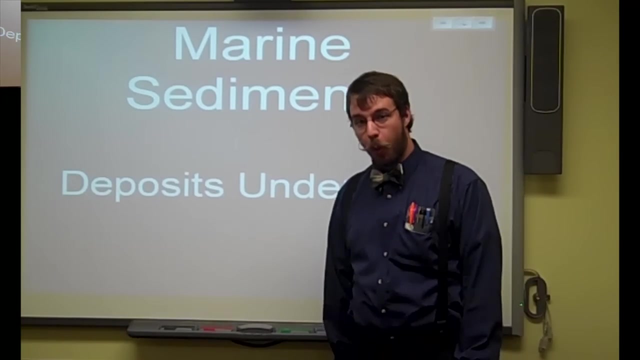 All righty boys and girls, thanks for tuning in on flippity, flip flop, flip class, the flipping class for Monday. I know you guys just had a test and you're probably like, oh, I have no idea how I'm going to do this stuff. But don't worry, I'm going to keep it, you know, mostly kind of short. Just a little introduction to the marine sediments. So, marine sediments, those are obviously sediments that are found, you know, underneath the water, in the bottom of the ocean area, in the marine regions. 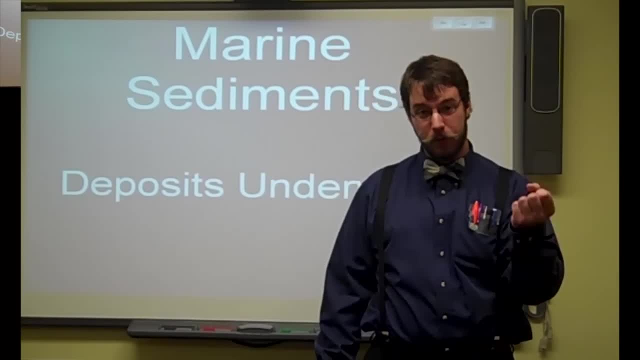 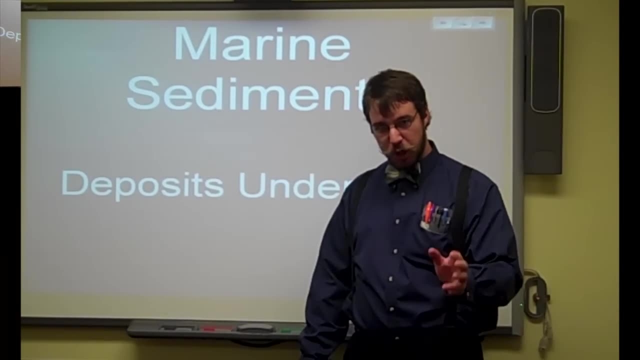 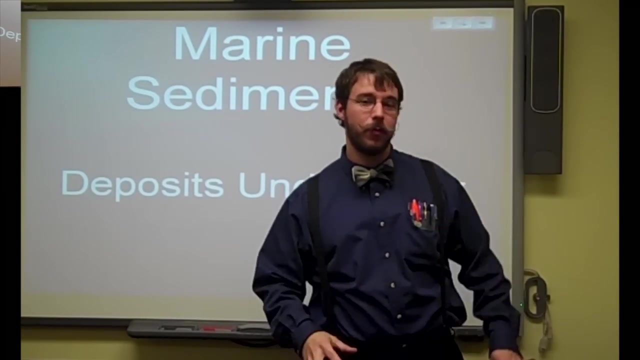 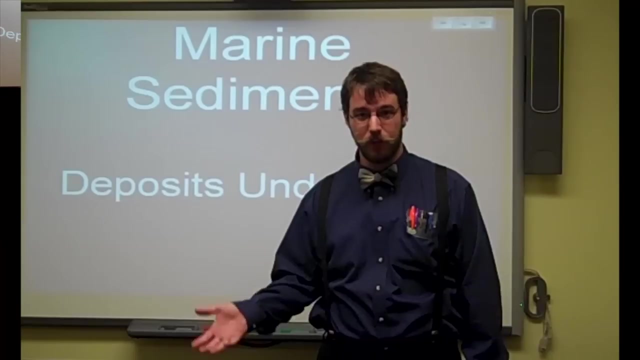 And what's really cool is based on the types of marine regions, like those three that we talked about. from the test we're talking like the continental margin, talking about the deep ocean basin, talking about the Midoshen Ridge- you can actually see different types of sediments common in those different areas. But what's really cool is, based on the types of sediments found in those areas, you can actually tell the geologic history of that area, as well as the history, the biological history, the history of species diversity, the history of evolution. 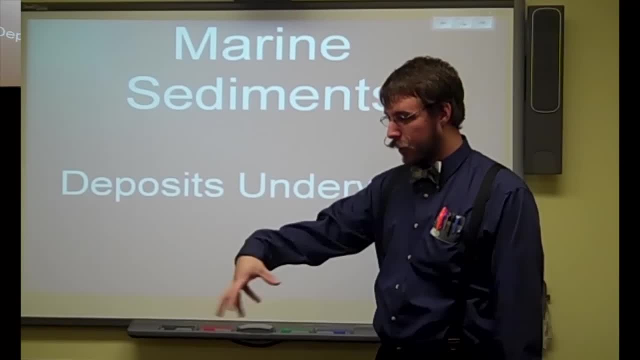 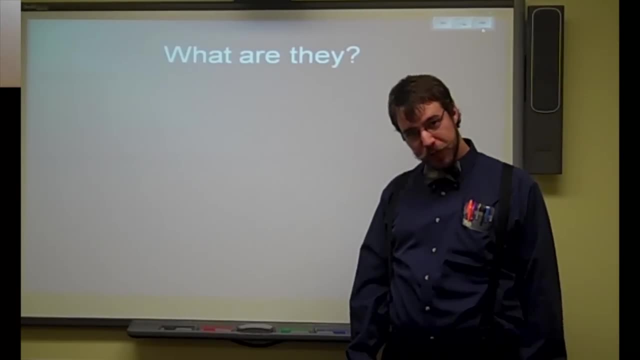 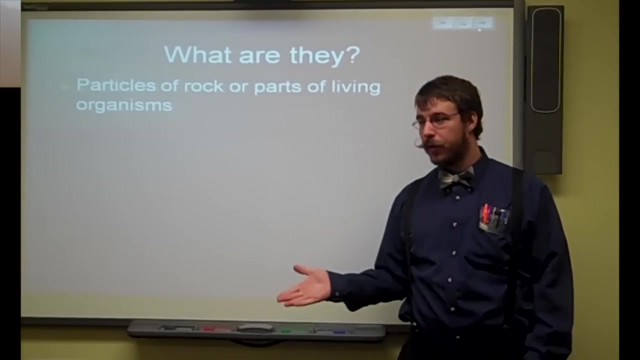 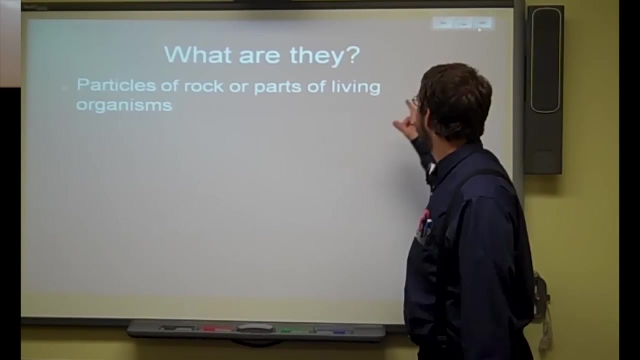 It's a really, really awesome thing. Lots of information is stored at the bottom of the surface, mostly covering the abyssal plains, So let's get into it, shall we? First things first, what exactly is a marine sediment other than you know? a sediment that's sitting at the bottom, Literally? what it usually is is particles of rock and other organisms. You know they're probably not living anymore, but they used to be Used to be parts of living things stuck down there and they're deposited away as of here. This is special. 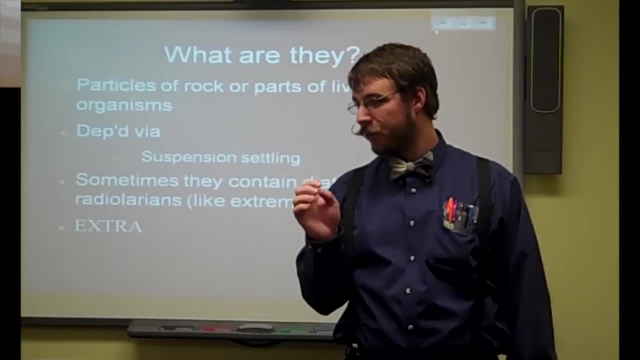 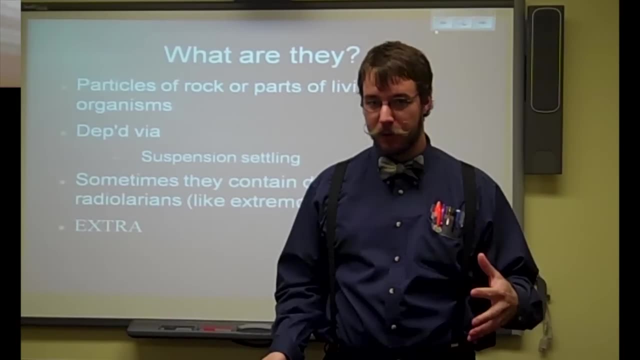 Now, sometimes they can contain little tiny protists called diatoms or radiolarians, and a lot of these are extremophiles. So we find some really cool ones up on the continental shelf in tropical waters, but we find some really awesome ones as you get closer to the Midoshen Ridge. 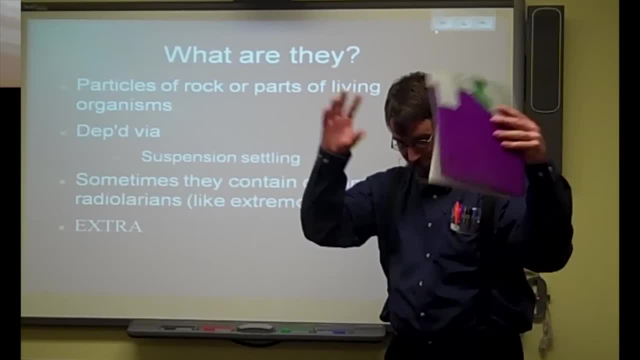 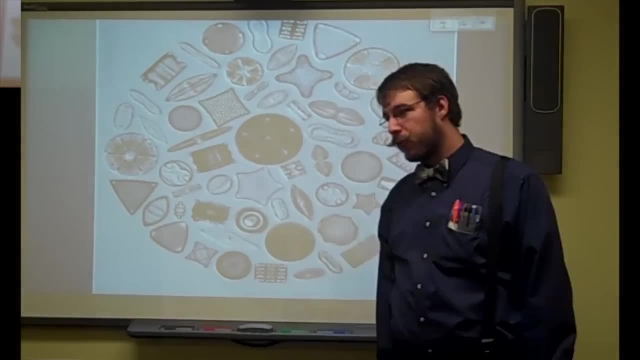 The problem with the Midoshen Ridge, though, is it's got, like you know, the lava coming out all the time covering all the really cool sediments, But there's still some goodness in there, So let's look at a picture. It comes right out of your textbook. 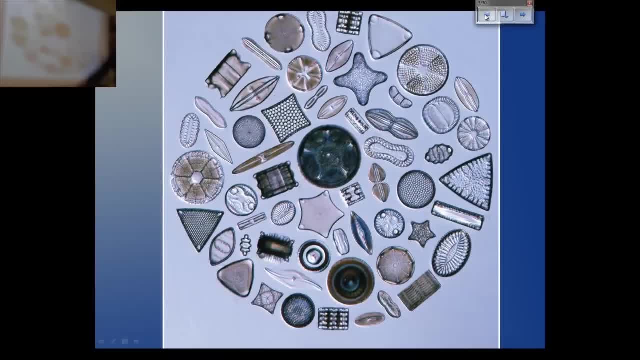 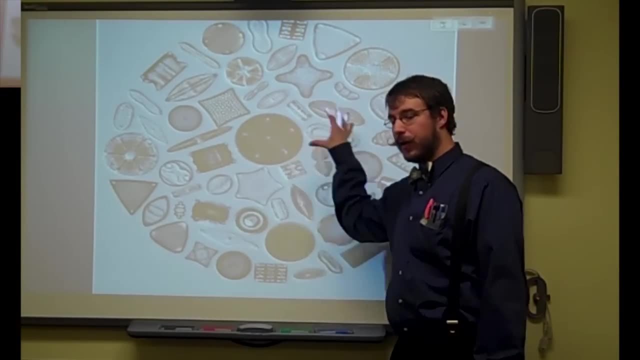 It's got microscopic diatoms and radiolarians. You can see that some of them have some really cool patterns of symmetry. These are really- I mean, they're just beautiful. And we have a bunch of these marine sediments that Mr Fry actually collected from all over the world that we're going to get to dig through and see how many of these you can find in there, which is really kind of cool. 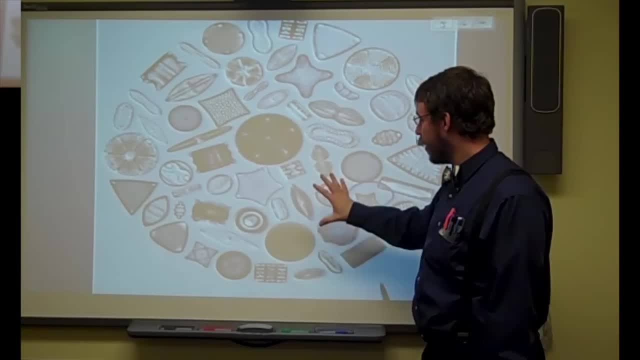 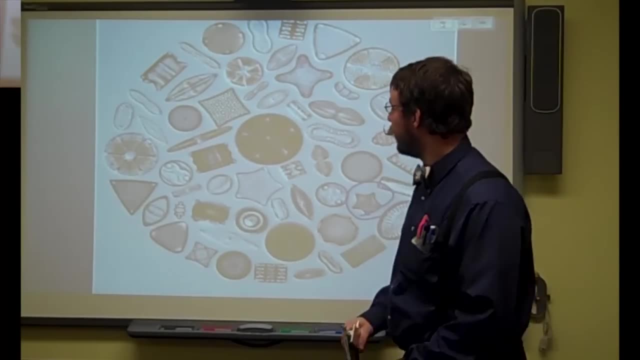 Literally, these are pieces of sediment. What's neat is they come from microscopic like shell parts of microscopic protists and other teeny tiny organisms that I mean you would never see. see, but they're also a hundred percent rock, which is weird. so the types of 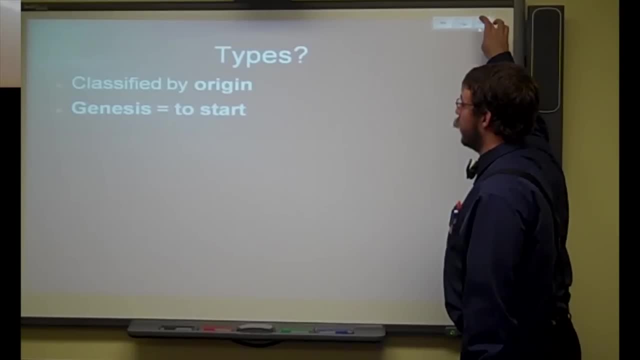 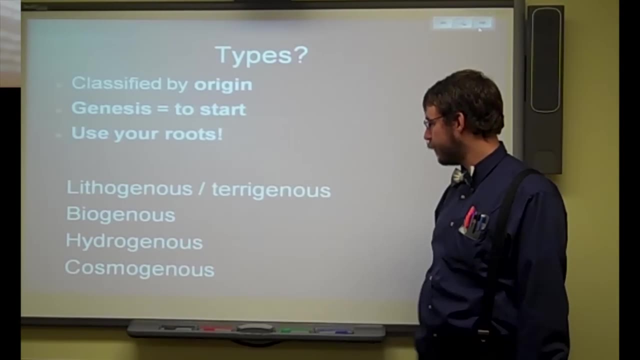 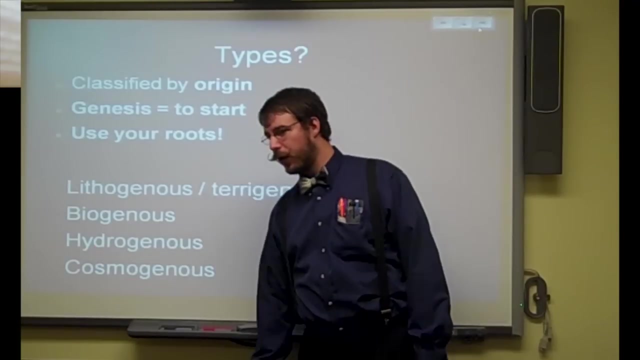 sediment are classified by the origin that they come from. they all have the word Genesis, which means a start. so then you just throw in your root words. there's lithogenous or a terragenous that you know started at rock, started at land. biogen is started as a living thing. hydrogen is started in the water. okay, 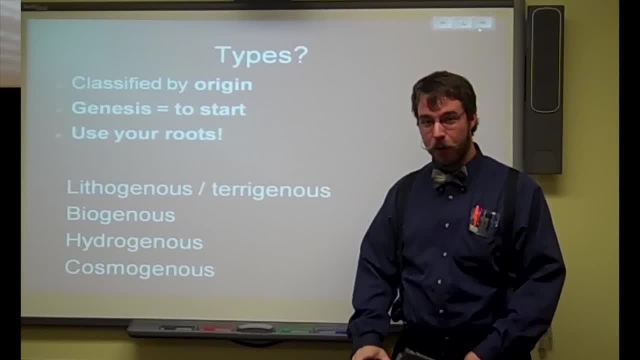 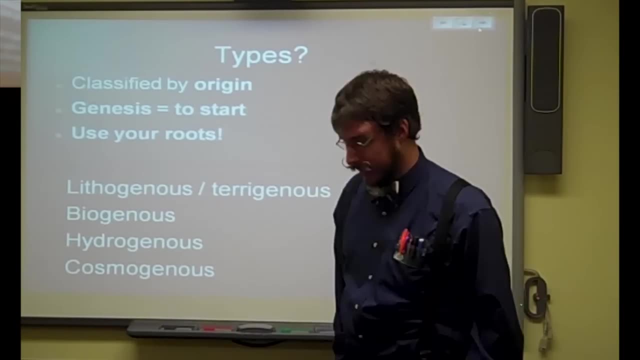 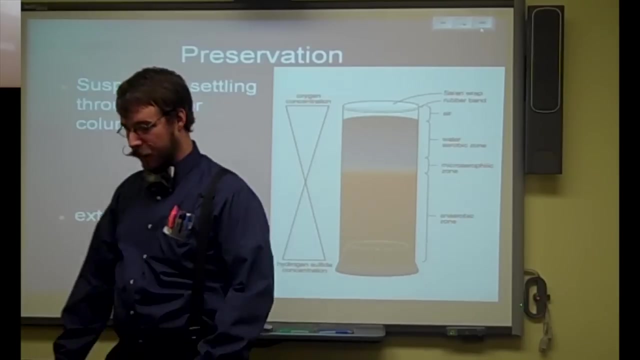 that one's weird. we'll get to that later. and then cosmogenesis- Cosmo- not talking about Cosmo Kramer, I'm talking about from outer space, man like meteor is and stuff, and alien deposits. literally now all these are, like we said earlier, deposited is the suspension. so what is really cool is most of the 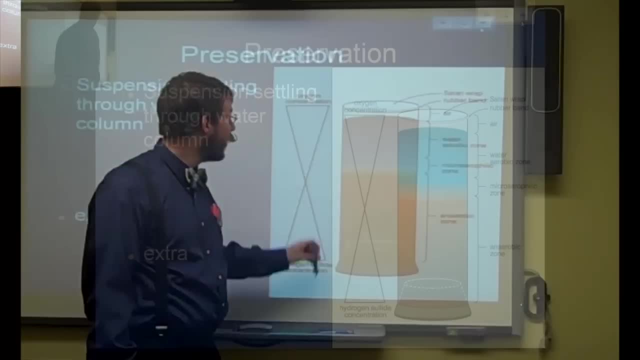 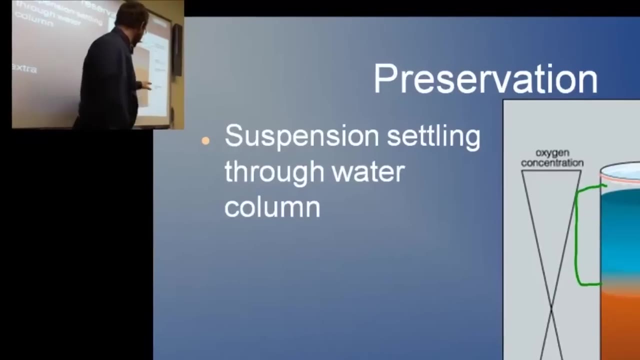 sediment because it's so fine, because it's so microscopic. it's mostly hanging up here in the water region and it can actually take on average ten to fifty years in the water, so it really is a really good idea. and then there's the years for it to settle to the bottom- just not even talking like for it to. 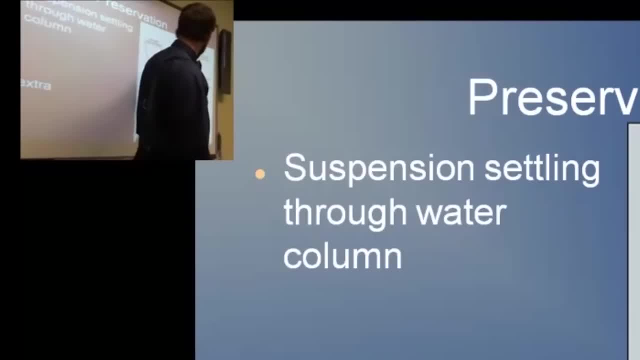 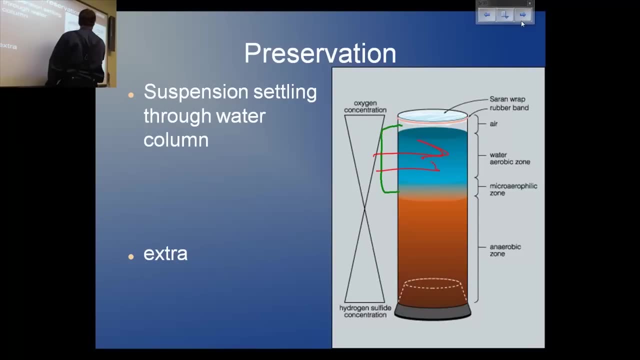 turn into sediment. I'm talking just for it to be deposited from here to there could take 10 to 50 years, and because the ocean has no currents and stuff in it, a lot of these sediments can actually travel up to 22,000 kilometers, which is 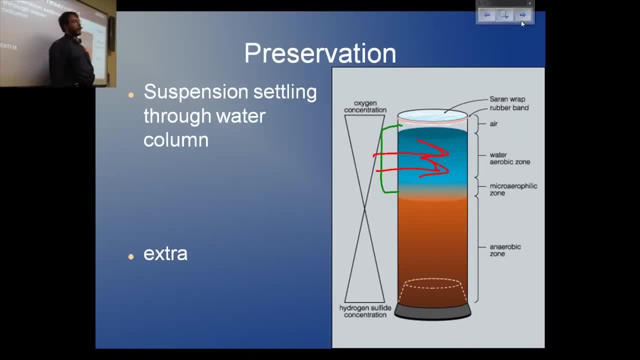 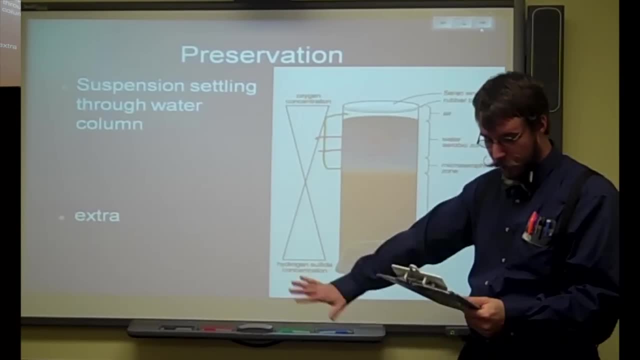 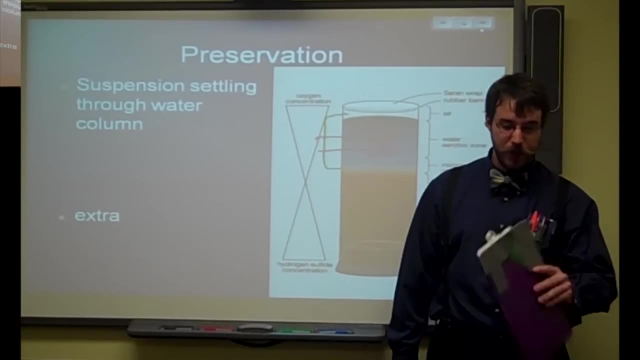 just the preposterous amount of space to cover so you can find things that came from the land really out in the deep ocean basin because they can travel those great distances. now it's really cool is there are some sediments that are really, really heavy. the most heavy stuff is actually feces. yep, feces. 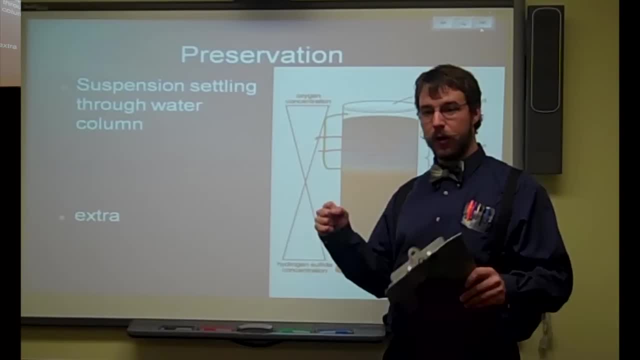 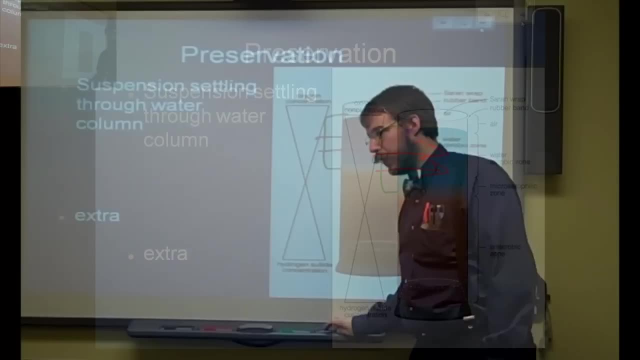 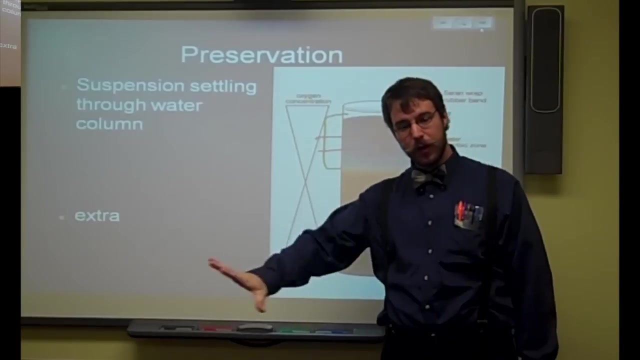 sediments, and especially ones from animals that are eating algae or eating produce, that are up here a little bit higher in the column and those will sink to the floor pretty quickly. we're talking about a 10 to 15 day descent to the bottom, so it's still, you know, you can get a little bit of movement. remember the. 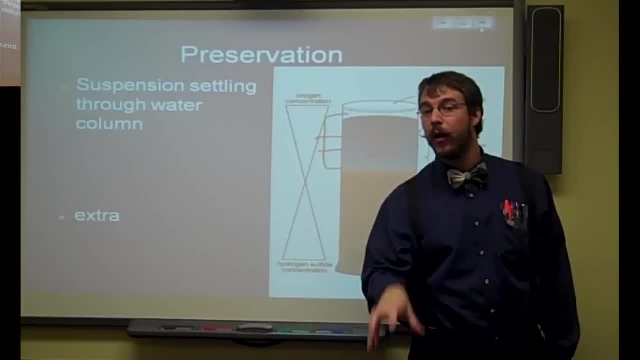 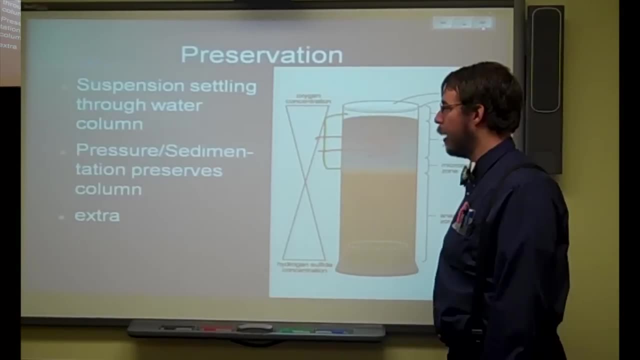 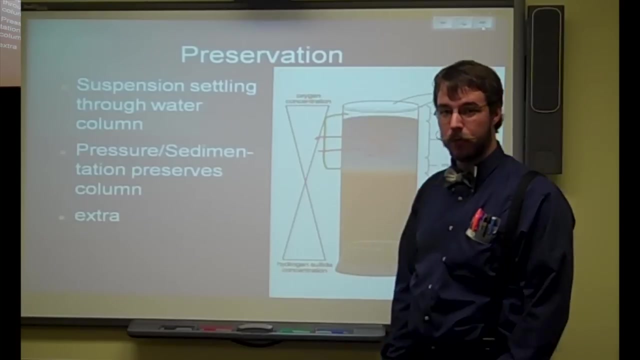 heavier the sediment, the more likely that you'll find it right in that area. the more dense the sediment, probably the faster it will sink and the less time it'll be hanging out in the water column. what's really cool is the pressure that the ocean is under actually helps to preserve exactly how the water column. 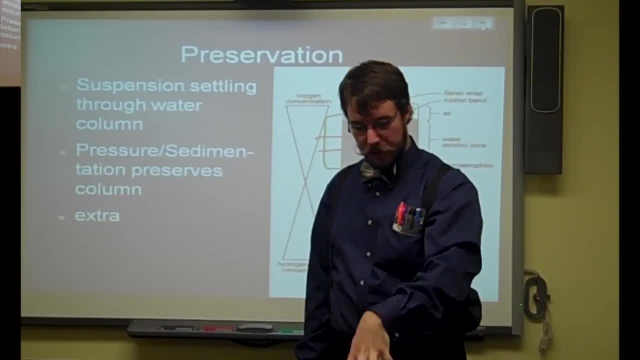 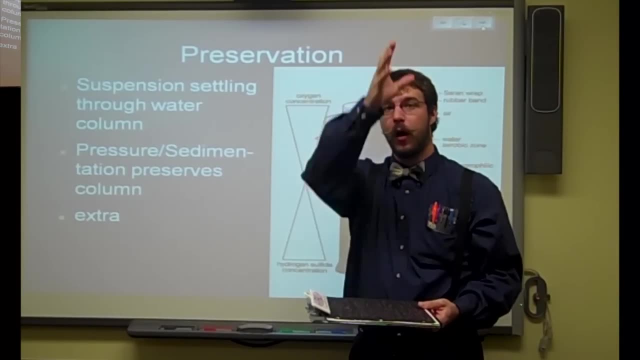 looks so we can actually see like a snapshot when you get into the like. if this is our stuff, if we get into the ocean floor and get into the sediment, you can actually see a snapshot of the sediment and you can actually see the the column of water directly above it, exactly how it would have been once upon. 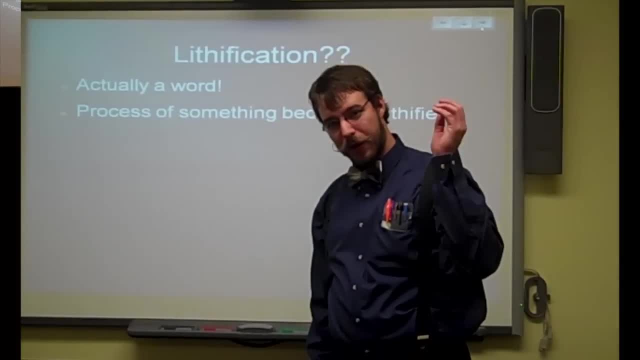 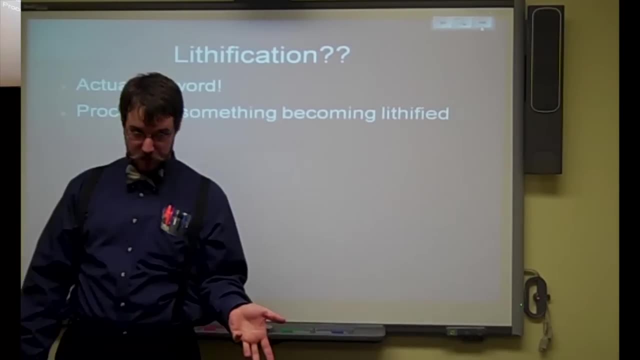 a time, all right. so what actually happens is then what it has been deposited. it goes through this process called the lithification, which is literally, well, the process of being lithified, which is literally the process of stuff that was not a rock being turned into stuff that is a rock like if. 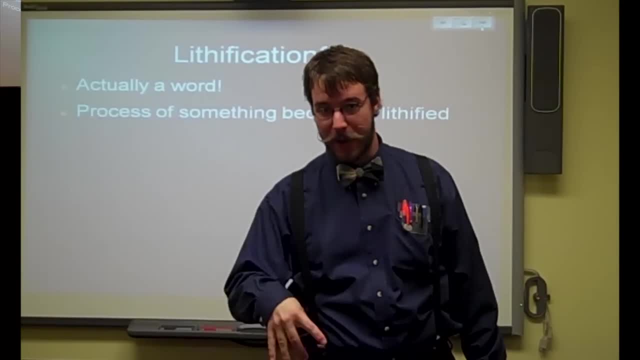 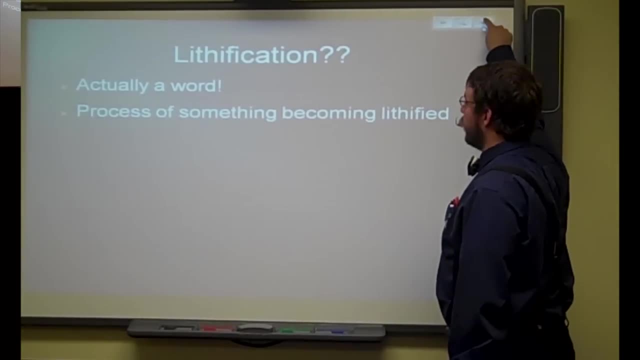 I went down to the bottom of the ocean, became lithified. I would be a rock now, not like a mr Patterson, but more like a statue of mr Patterson. a big part of that is due to the pressure but also different chemical reactions that happen in the sea floor. they become sedimentary types. 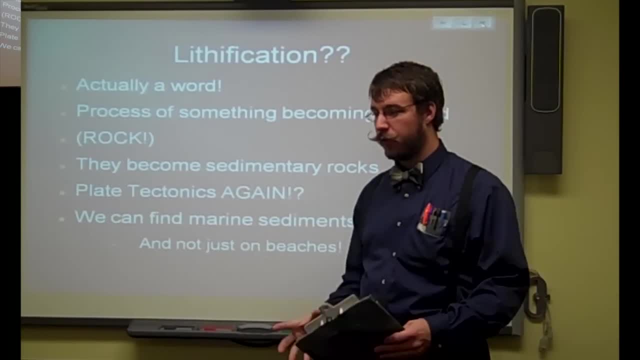 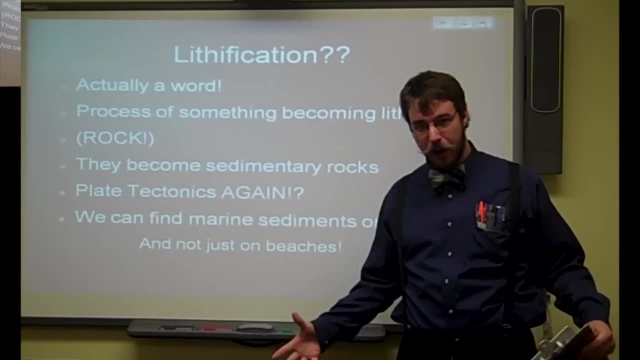 of rocks. plate tectonics can play a big role. you can metamorphose some of those, you can bury some of them. but what's really neat is we can actually find, because of uplifting, because of the whole plate tectonic, that whole like continent moving idea, we can actually find marine sediments on land and I'm 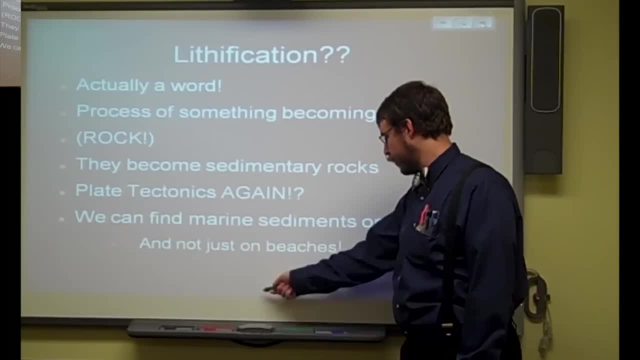 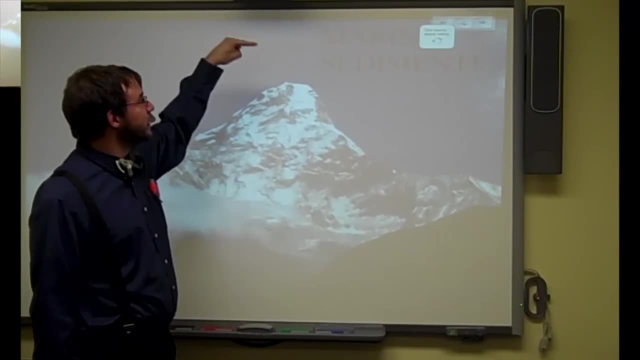 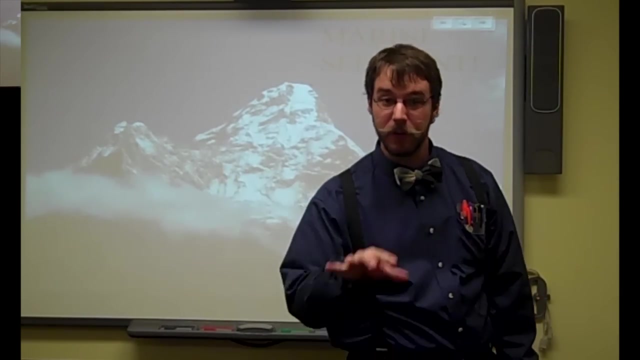 not just talking like a beach sand. obviously that's gonna be very sediment. all over is a place sediment, sediment sediment. I'm talking marine sediment on tops of mountains. I mean that's the whole reason why, like we have shale here in Ohio, that's marine sediment. those are sedimentary rocks. 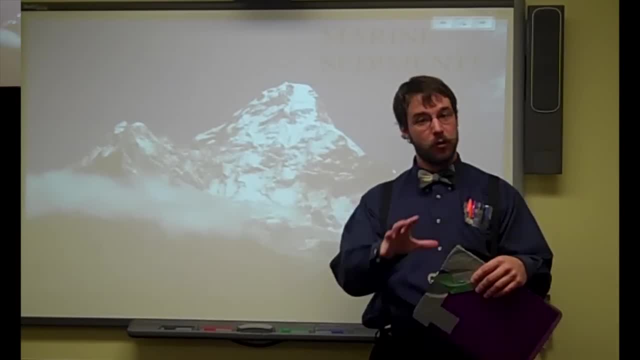 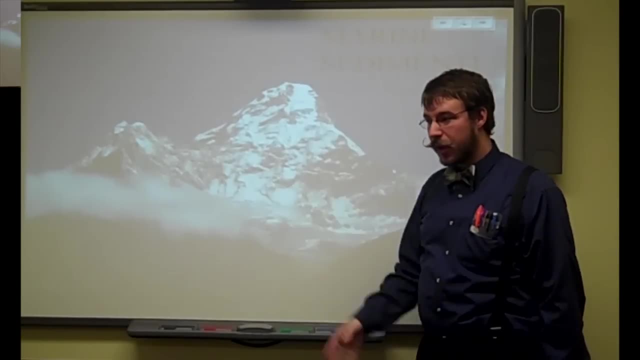 deposited by the ocean. it's full of all these like biotic creatures and that's what actually makes a natural gas and the oil and the other stuff that we've been going after for all these years. I mean up up here, not even getting close to them. that ocean up there it's awesome and what's really kind. 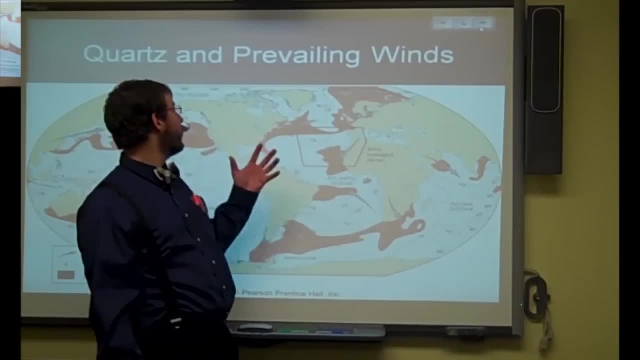 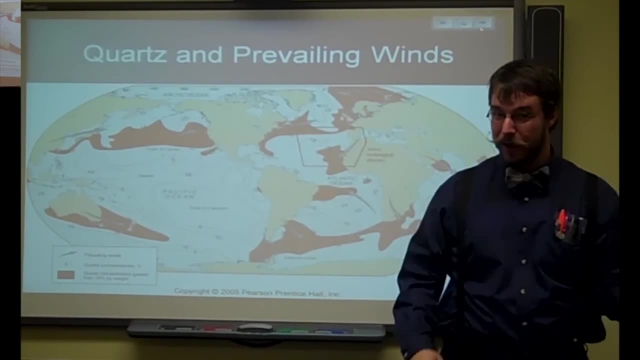 cool, And that's just the big stuff that got deposited. That doesn't even account for stuff that gets blown around. So here's a really good picture that actually shows you a prevailing wind sending teeny, tiny pieces of quartz. Now, quartz is not very water soluble- not really at all. 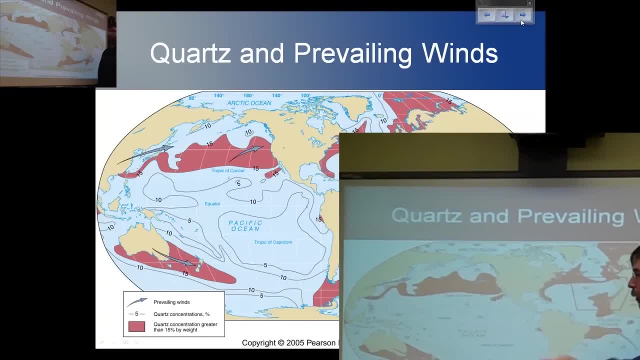 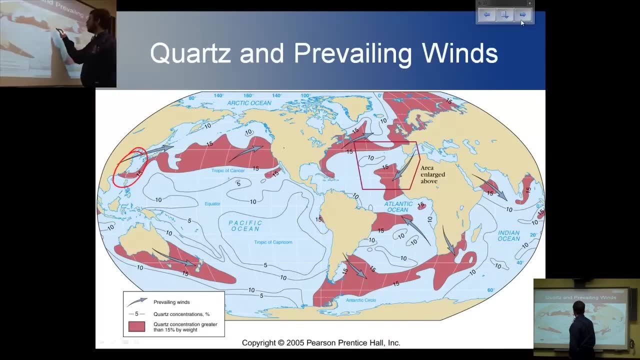 only dissolves in really, really hot water. So you know, these tiny particles and this is just stuff that's just been carried by the winds, Like literally, you can have sediments from over here in the Americas that can be carried by the wind or, sorry, over here in Asia that can be carried by. 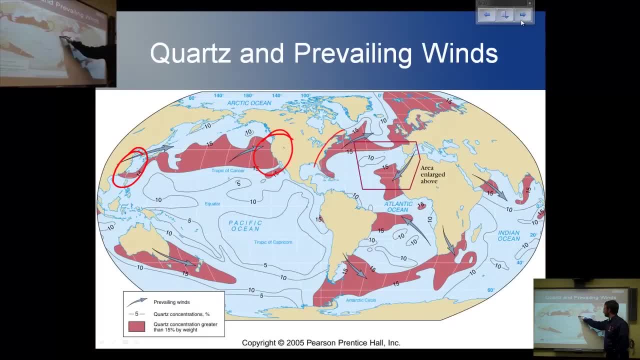 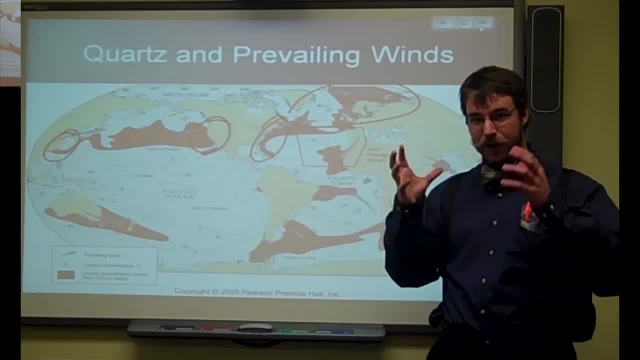 the wind and deposited on the West Coast. And the same thing. here we've got the East Coast of America and we can deposit all that up in over in there. I mean, this is stuff that's from the land, It's terragenous sediment that's carried by the wind, And then you can imagine how far it's. 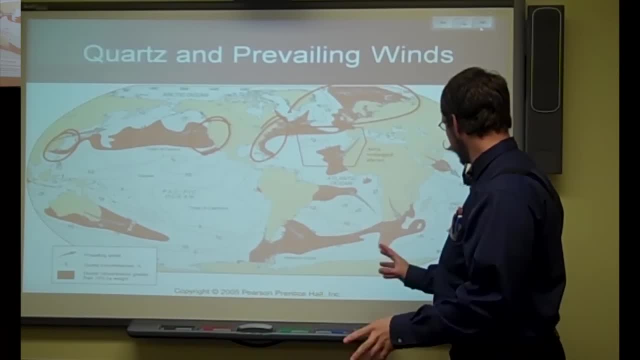 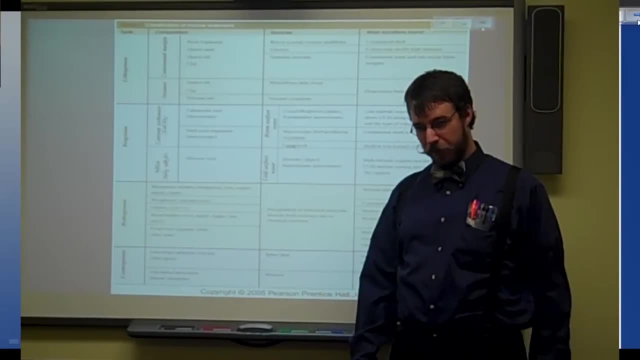 going to be carried once it actually gets into the ocean. So it's a really cool and complex situation. Here's a table from the book. This is table 4.1 in the old edition of the book. I'm assuming it will be table 4.1 in the new edition of the book, But if not you might want to check. 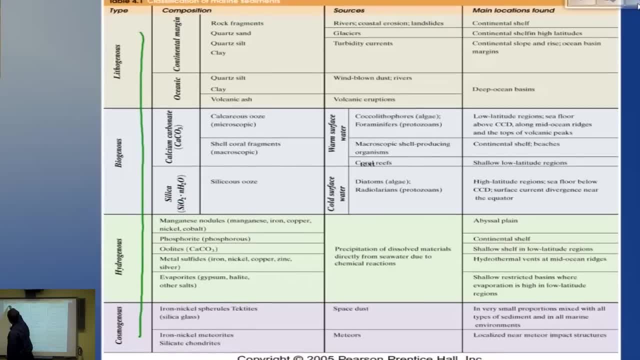 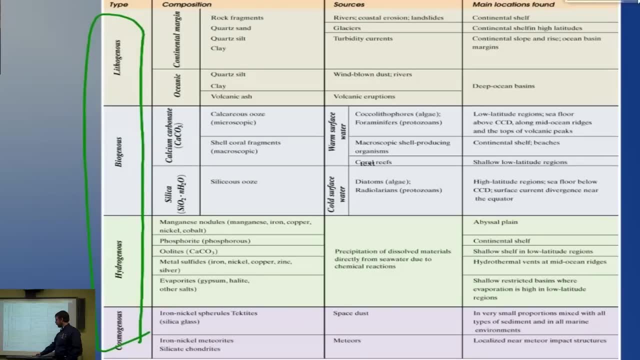 it out. It's definitely going to be chapter 4 because that's the sediment chapter, But it actually breaks down the different types of sediments for you really nicely and then gives you a plethora of information. You definitely have things you need to know. You need to know. 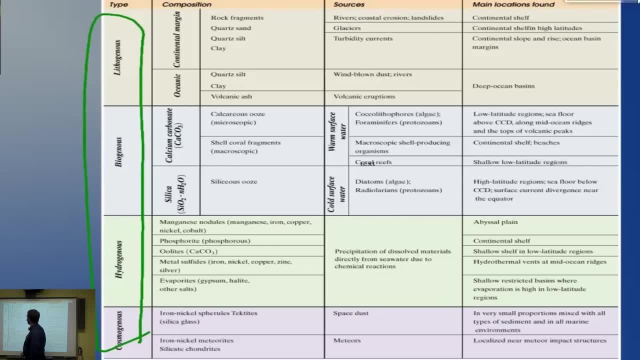 specific types of sediments. You definitely need to know this first column. You want to know what kinds of rocks, et cetera, they're made out of. You need to learn to use words like ooze, microscopic, macroscopic silicates, stuff like that, That's, the elements that have silicate. 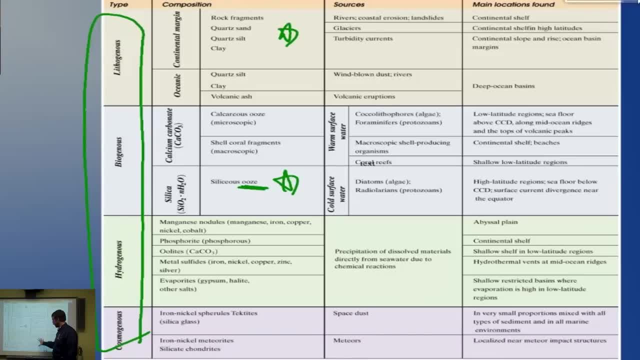 in them. by the way, You're going to need to know the sources, because when you know the sources then you know where those things came from, Then you know the geologic history And then you want to know approximately where they're found. So really you pretty much need to know this whole. 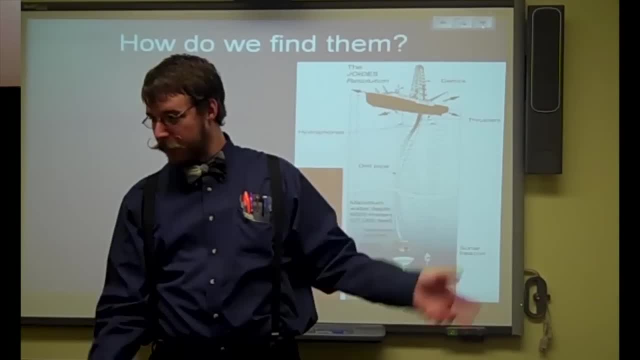 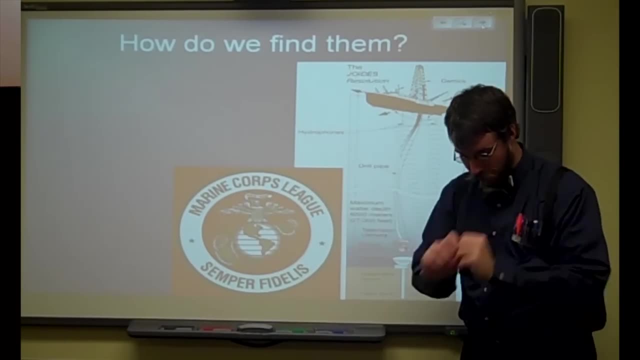 table. So you've probably been wondering to yourself: with all the blowing of the sediment all over the place and the craziness, and then the suspension settling and the 10 to 15 years of dropping to the bottom, how do we find this stuff? Well, 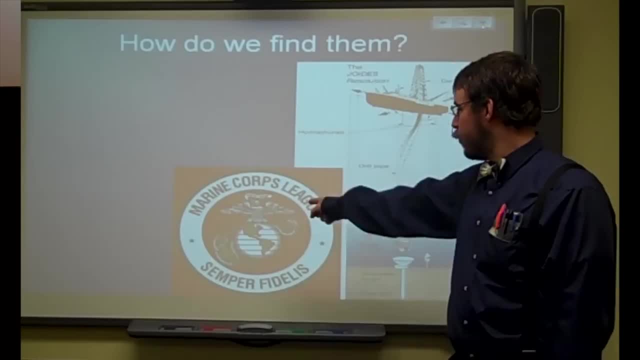 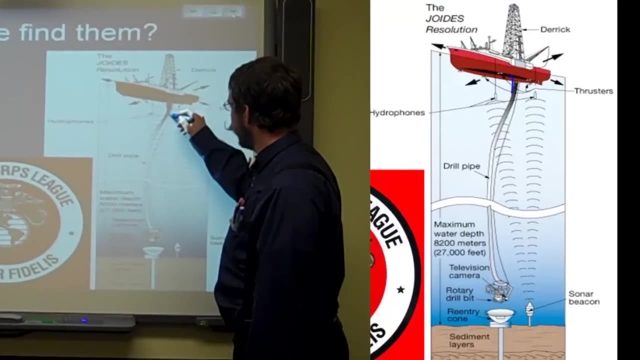 we look for Marine Corps- And I'm not talking about like the USMC Marine Corps, I'm talking like we send a ship out sort of similar to an oil rig ship And what we do is we send, like a big old hose, down to the bottom, Down to the bottom. this is showing that it's cut off and 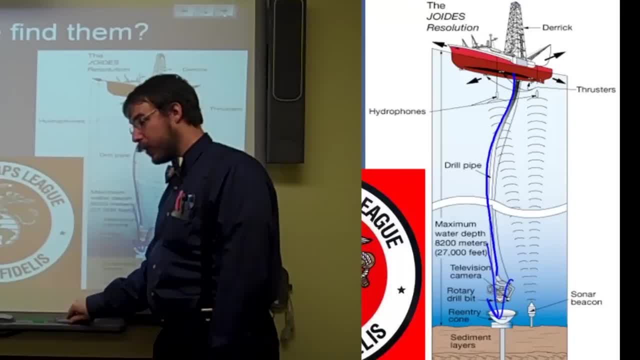 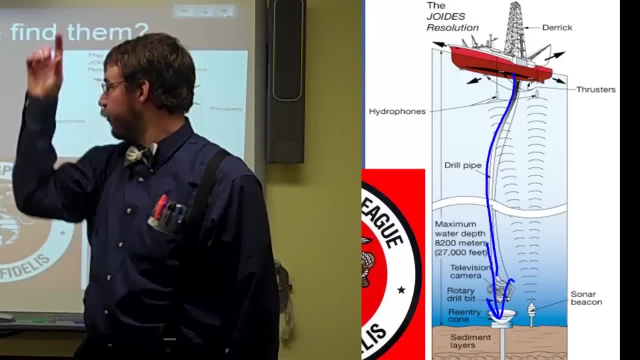 drawn out to scale And we stick it into a hole And we literally have to drill on it. It just drills down, grabs a chunk like a column of sediment. It just pulls it all the way back up to the ship. So literally we send down, drilling to the bottom of the sea floor. 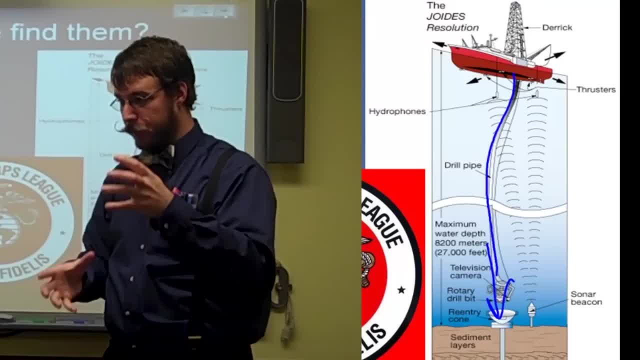 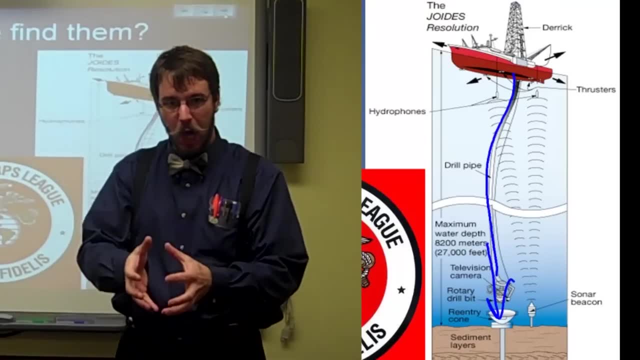 to investigate what we see And we're looking for cores And literally it's like you know, have you seen like those apple cores? You can stab an apple and pull out just the core And it's like this cylindrical column of apple that you don't want to eat because it's got the nasty. 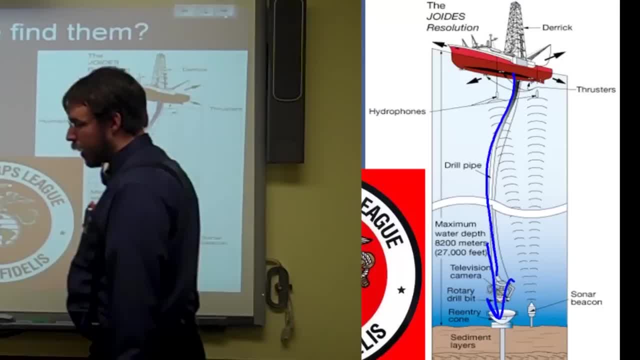 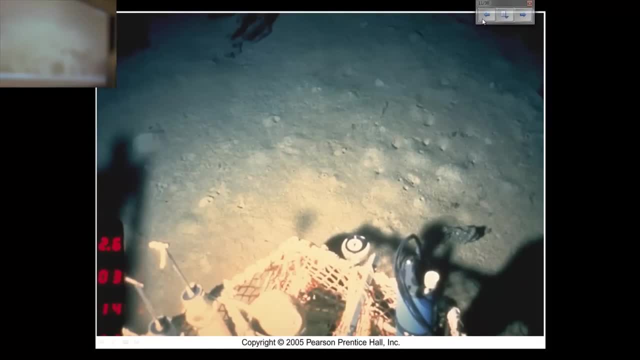 core in it. That's the same idea. You just stick it in there And we get this nasty core of marine sediment, And then you can look at it and see what's in it. So here's a picture taken from one of the cameras. This is at the ocean floor. They're going to pop right into that little loopy hole. 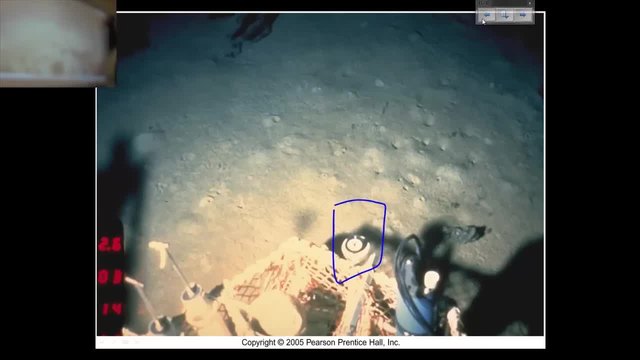 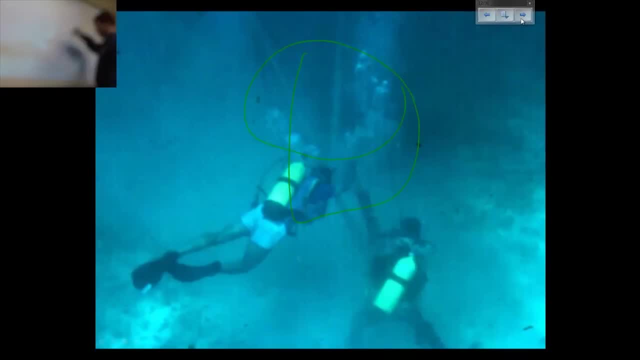 Right here And they're going to go in and they're going to get themselves some sediment. Here's another picture of some deep sea divers. They're doing a little bit of maintenance on the big old drilling thingy which is right over in this area. here And again they're getting some sediment. 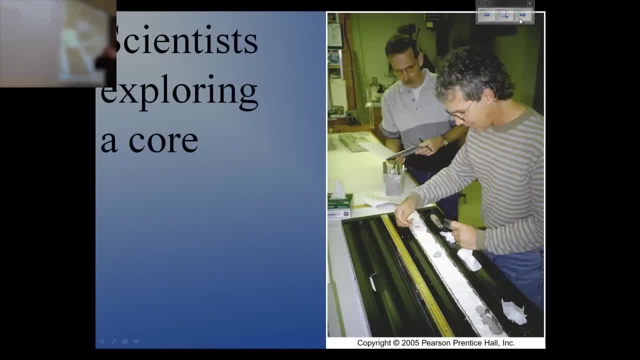 And then when you get the sediment, literally this is what they do. They take the sediment. It's preserved in these like metal tubes. They open the metal tube And then they meticulously pick through it for like ever, and see what's in it. They sometimes burn some of it, break it up into. 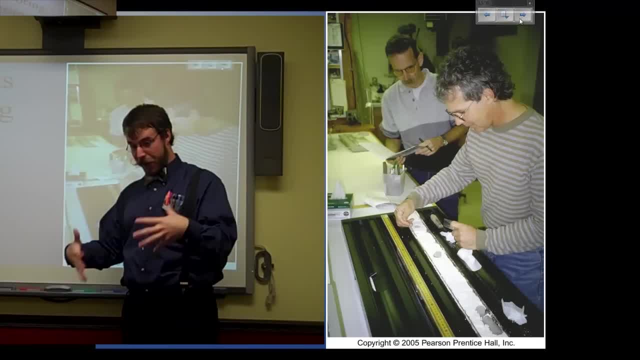 little bits, destroy it by doing chemical destruction, And then they take the sediment, do a little test and figure out. you know just what was going on with the ocean floor. What's really kind of cool is you can actually see due to some geological stuff. 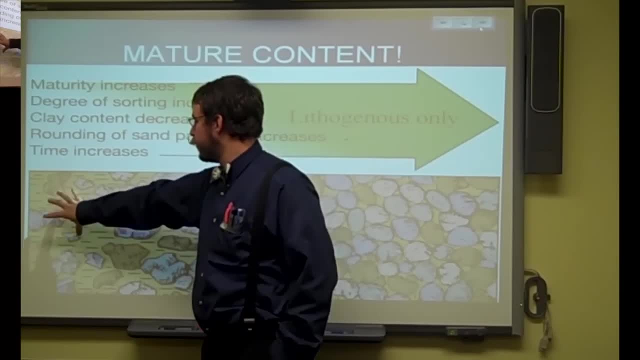 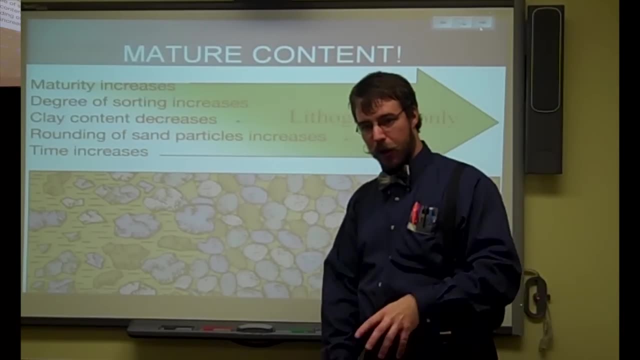 you can actually tell the age of the sediment based on: is it really chunky and stabby or is it smoother? Is it better sorted By sorting? think of our graded bedding. Are all the little things with other little things and the big things with other big things, Or is it all? 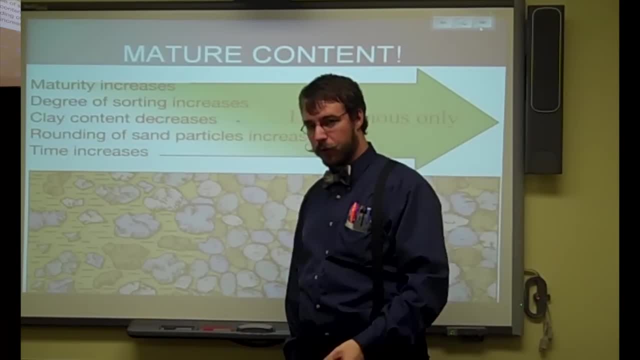 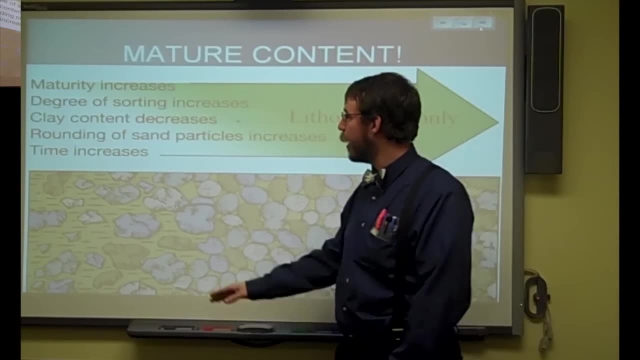 kind of mix-mashed in together. The longer a sediment goes and sits at the bottom, the rounder it will be. the rounder it will be, the better sorted it will be. In addition to that, it also eliminates the silicates, eliminates the quartz elements and turns them into clays. 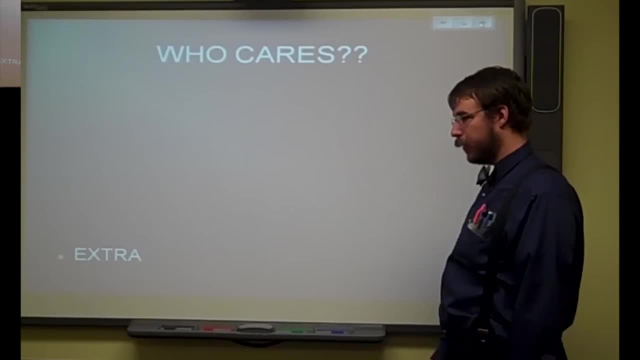 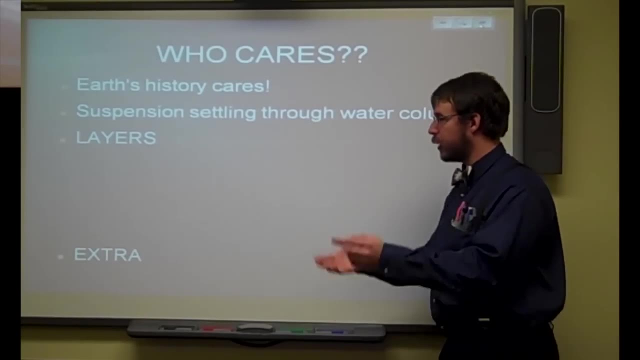 which is just, you know, microscopic mashings of rock. So the question is: you know who cares? Well, you should care, because Earth's history cares and you live on the Earth. It's a special sediment, It takes a very long time And, like we said before, you can literally see. 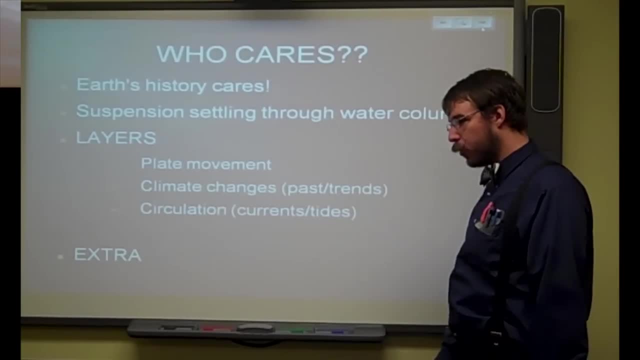 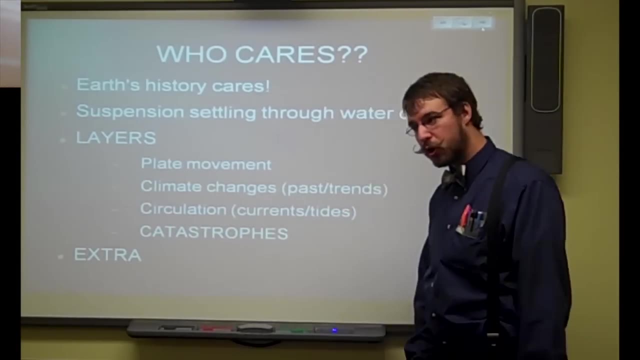 all the things that have been happening inside the world part area. Very important because it gives us more evidence for my favorite stuff- theories to protect times. But it also has been showing us evidence of past and present trends of the climate. It's not just about the glaciers. 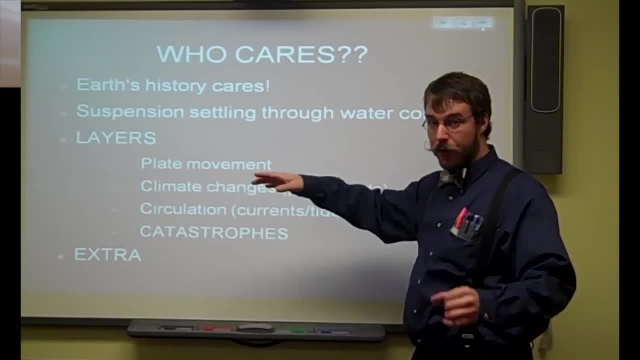 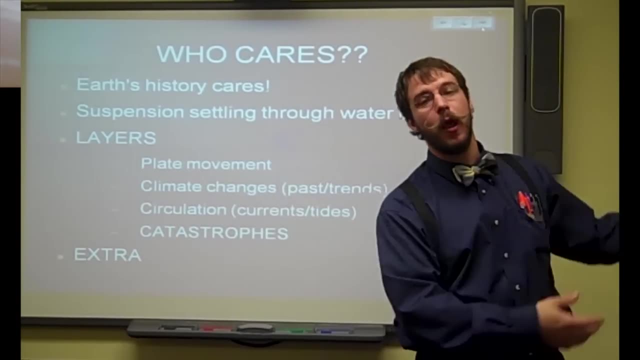 it's the ocean floor of people. seriously, We've actually seen evidence of not just our climate, past climates, three, four, five climates ago. We can actually track all the four ice ages before based on what we're seeing in the sediment cores, based on the types of rocks we're seeing, based 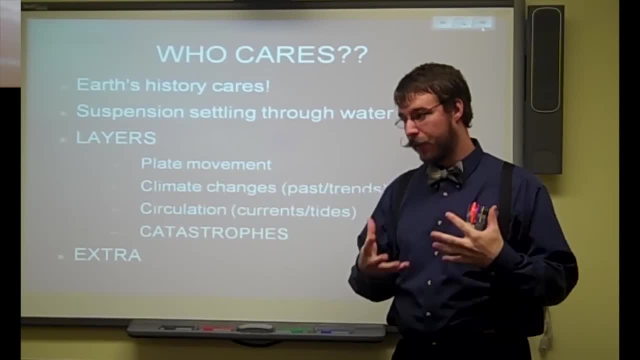 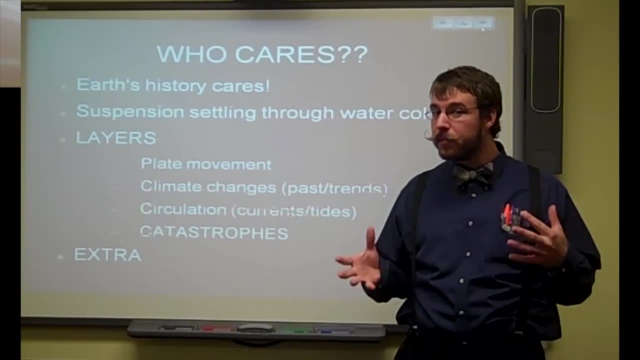 on the gases that are trapped in there and based on the type of life forms that we find in there. What's really neat? you can see catastrophes- I mean the marine cores associated with, like Mount Vesuvius blowing up are awesome- And you see all this really good data where you can track. 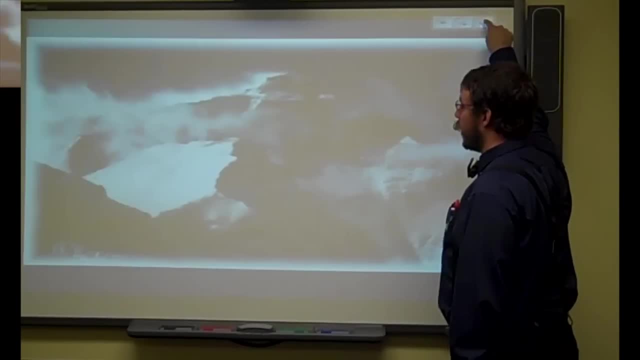 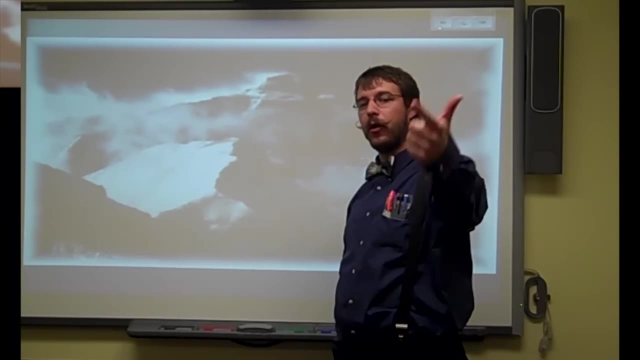 circulation in the ocean. I mean, you can just tell what's been going on with this, You can tell that this used to be ocean and we can tell what the climate was like, how long ago it was an ocean, what sorts of things were living there and how they compare to the things living in the ocean. 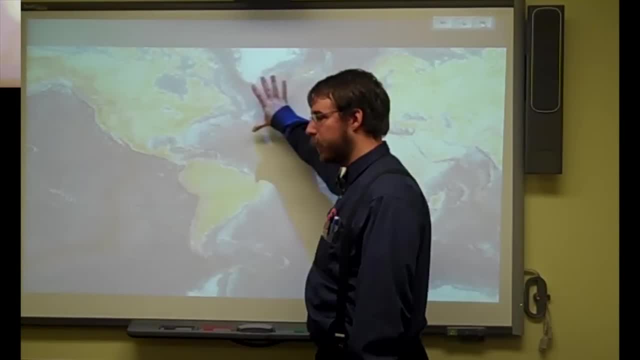 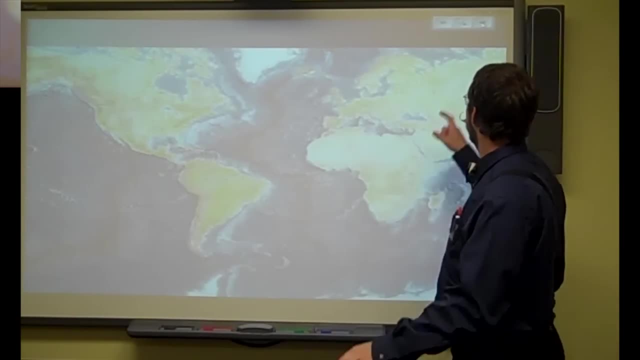 today, And so what that really does is it helps shrink this big picture of the ocean down to a smaller, manageable sizes that we can do quantitative data on and figure out you know what's been going on. I mean it's just, it's so awesome. It gives us not only an idea of the 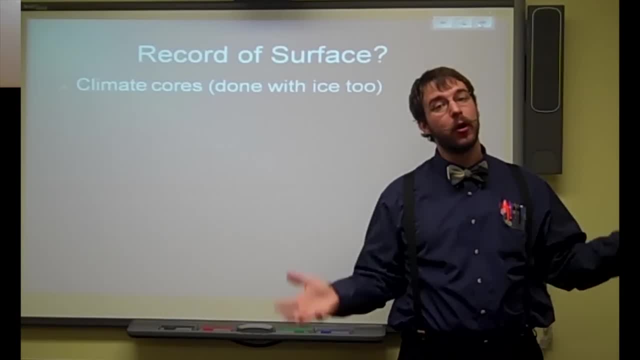 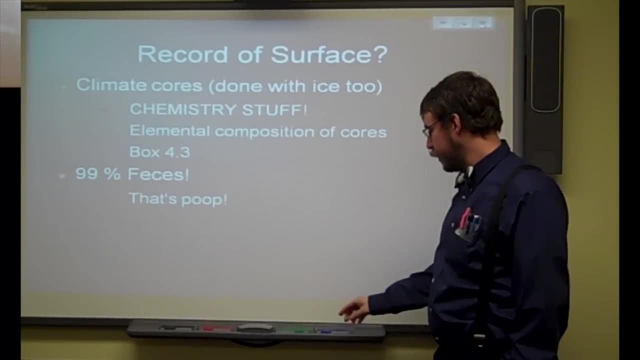 marine life, but it also gives us an idea of what was happening on the Earth's surface as well, which is pretty neat. You definitely need to read box 4.3 in your books that I know you guys totally took home. If you don't, you're not going to be able to read it, But if you did, you're going to. 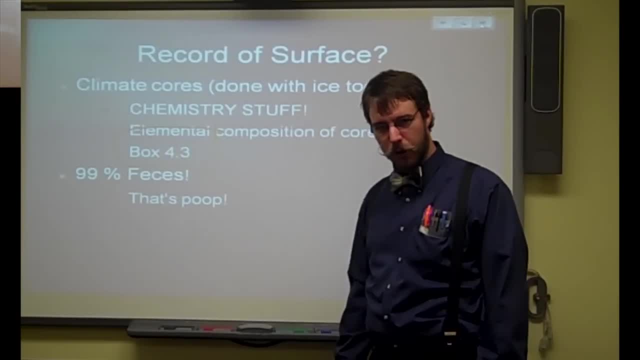 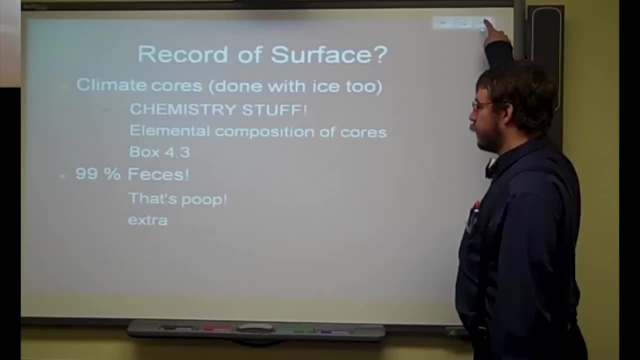 have it at home because I don't know. you put it in your locker because I don't know. you want to rip the book apart and then wood glue it back together. at the end of the year You could also come in and get one from my room if you need to read it during a study hall, And that boys and